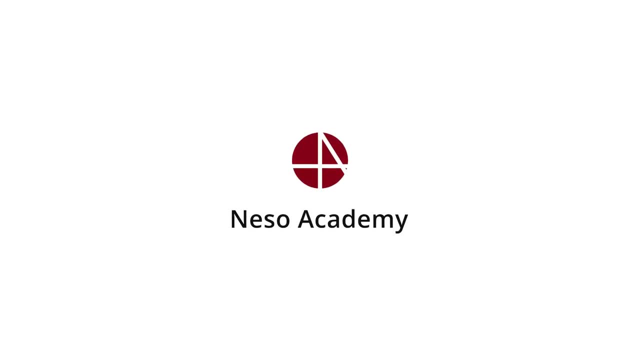 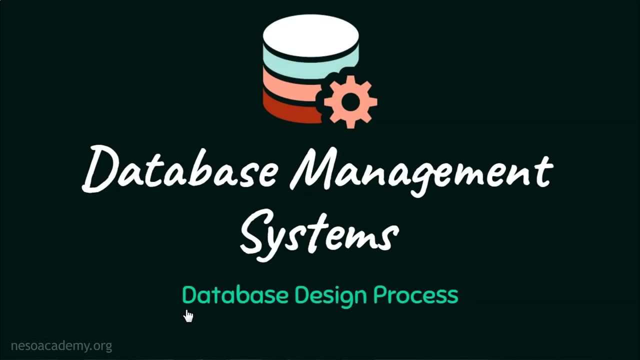 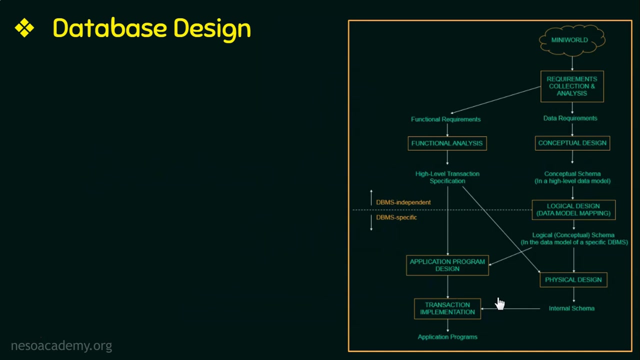 Hello everyone and welcome back. In this video we will be looking into an overview of the database design process. This is a simple illustration of a database design process. The first step in the design of the database is requirements collection and analysis. What is requirements collection and analysis? As the name itself suggests, database designers. 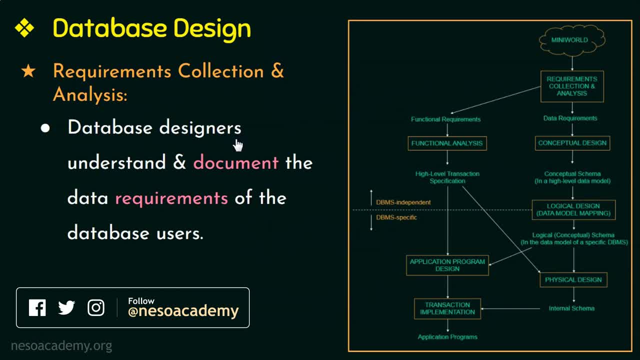 interview or ask the database users about their requirements and then try to understand and document the data requirements of those database users. The result of this step is the data requirements of the users written concisely or written in brief, or requirements. written in short, yet contains every detail and information. 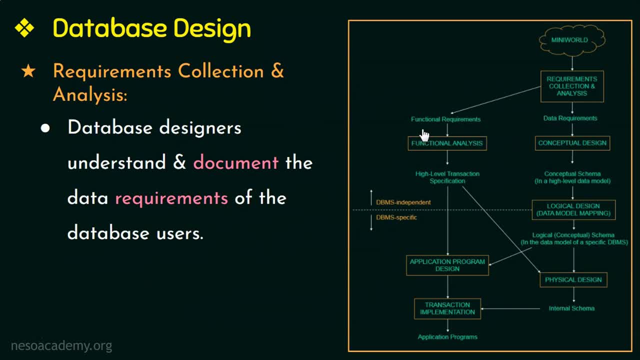 Along with specific data requirements, there are also requirements, collection and analysis, the user's data requirements, the functional requirements, also have to be specified. These functional requirements consists of user-defined operations that has to be applied to the database, and it could also include retrieval and updation of data. Once all these requirements are collected, 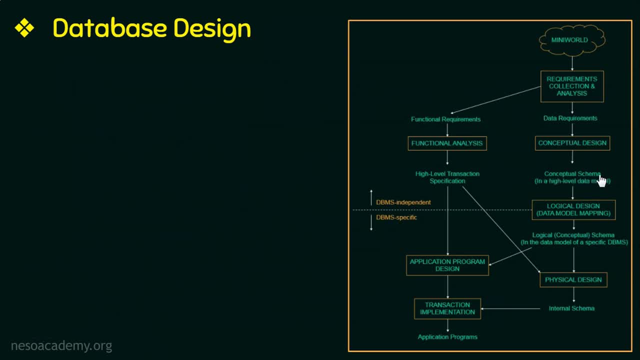 and analyzed. the next step is to create a conceptual schema for the database using high level or conceptual data model. We have already seen what a high level or a conceptual data model is. A high level data model is a data model that provides concepts close to the way how users 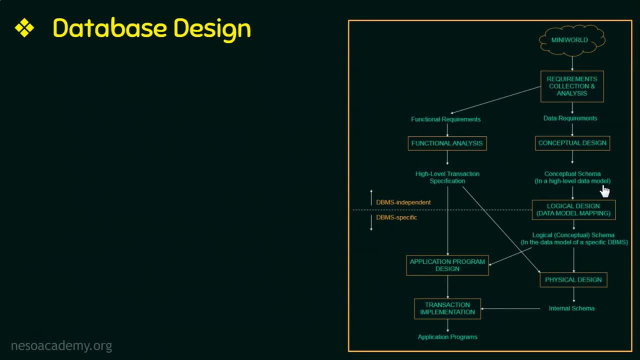 perceive data or how users see data. So, using this model, a conceptual schema is created and this particular step is called the conceptual design. This step is for creating conceptual schema. A conceptual schema is a concise or a brief description of the data, requirements and detailed description. 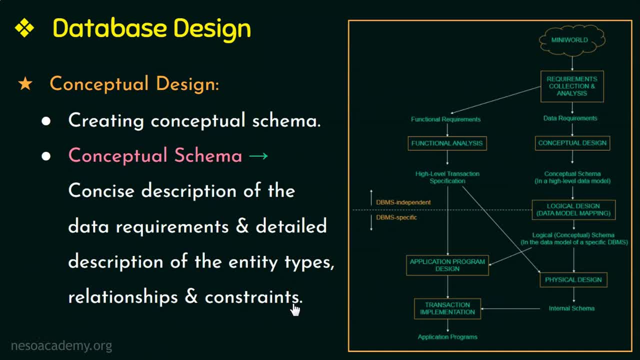 of the entity, types, relationships and constraints. You will understand this better with an example that we will be seeing later. As we saw, these concepts are expressed using high-level or conceptual data model and because these concepts do not contain the implementation details, they are easier to understand and 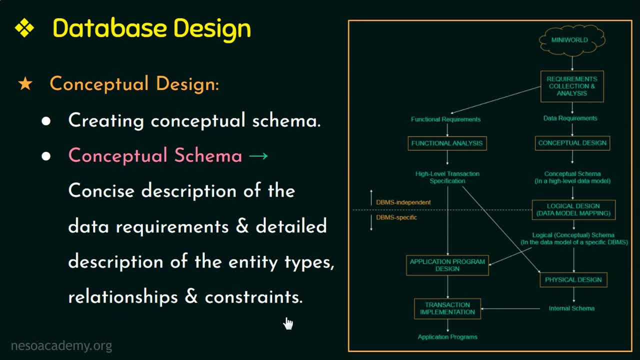 also, they can be communicated easily with the non-technical users. We saw that in the functional requirements the user-defined operations are specified. So during or after the conceptual design, basic operations are used to specify the user-defined operations that we identify during functional analysis. 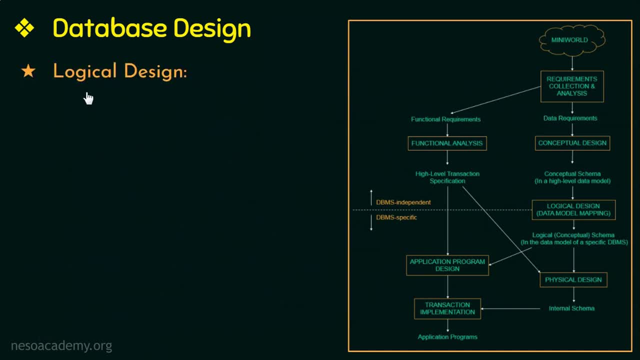 The next step in the database design is logical design. This step is the actual implementation of the database using commercial DBMS Like Microsoft SQL Server, Oracle, etc. Most commercial DBMS uses implementation data model. Again, we have seen what an implementation data model is in our earlier videos. So here the conceptual schema. 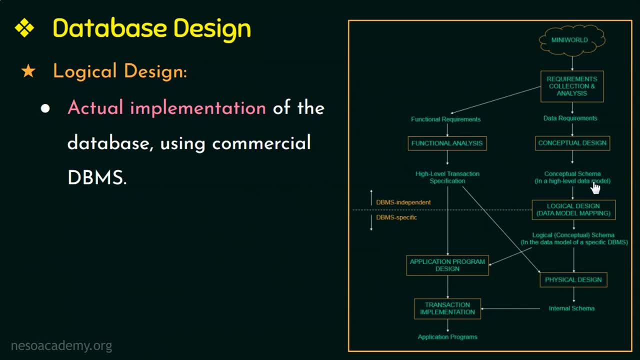 is transformed from the high-level data model into the implementation data model, and this step is called as a logical design or data model mapping. The result of this step is a database schema in the implementation data model of DBMS. So here we had a conceptual schema in the high-level data. 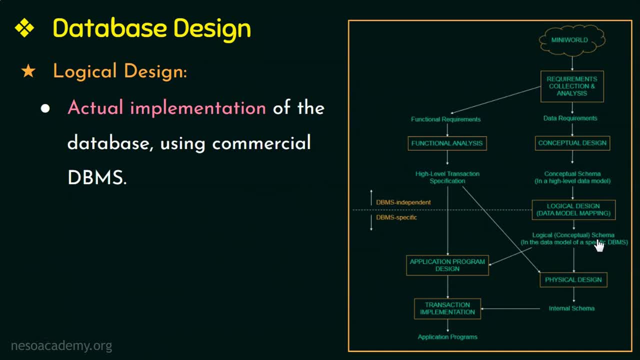 model, which is transformed to a database schema in the implementation data model. The last step is the physical design. In this step, the internal storage structures, indexes, access paths of the files are specified. Along with these activities, application programs are designed and implemented. 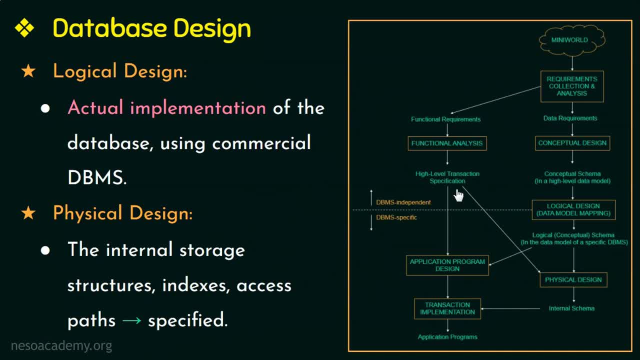 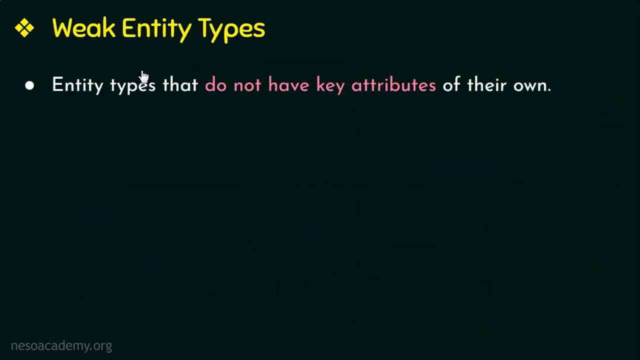 as transactions corresponding to these transactions. So this is a very simple overview of the database design process. Before we see an example of a database application, let us see what weak entity types are. Weak entity types are entity types that do not have key attributes of their own. In contrast to this, the entity types that have 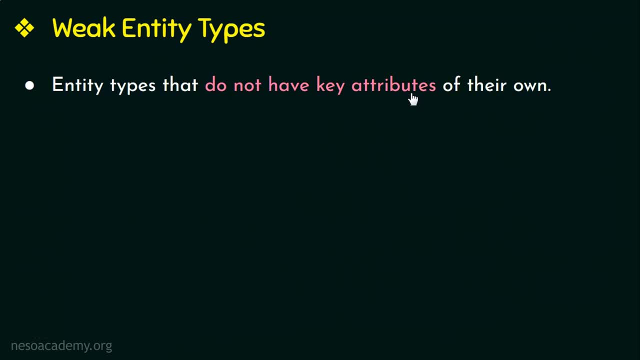 their own key attributes are called as strong entity types. The entities of weak entity types identify themselves by relating to entities of another entity type, And this other entity type is called the identifying entity type or the owner entity type. And the relationship between a weak 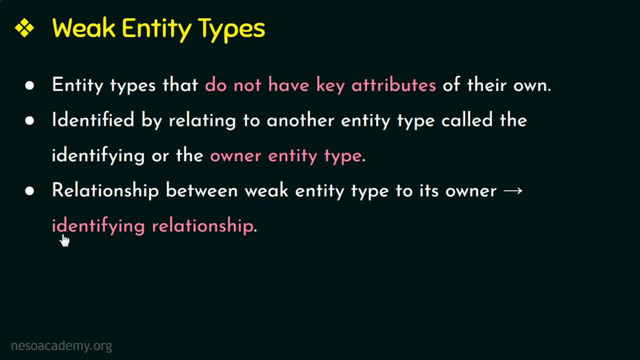 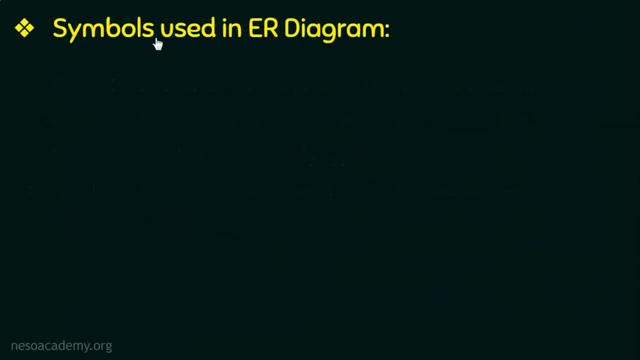 entity type to its owner. entity type is called the identifying relationship. So this is about the weak entity types. Now let us look into the different symbols that we use in the ER diagram. First one is the identity type. This is a regular entity type. We already learned what an entity is: It is a thing or an object. 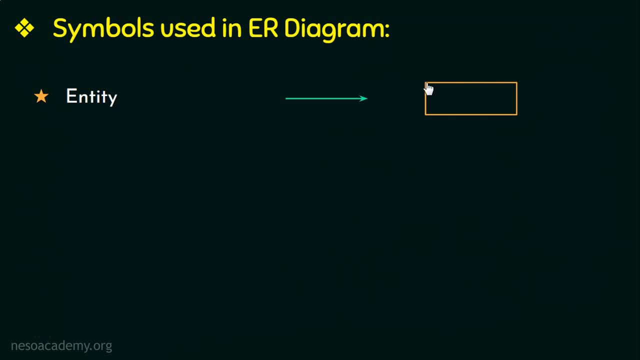 that has existence, and it is represented by a rectangle. This regular entity is also called as a strong entity. Next we have weak entity- We just saw what weak entity types are- and it is represented by a double rectangle. Then we have attribute, which is the property to describe an entity, and it is represented by an oval. 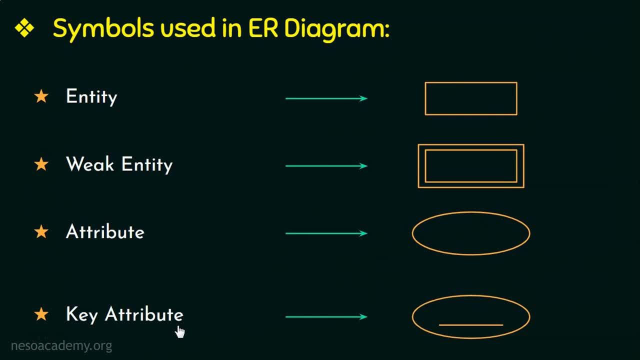 And a key attribute which helps an identifying an entity uniquely is represented by an oval with the underline under the name of an attribute that helps to identify an entity uniquely. The next symbol is the multi-valued attribute that contains a set of value for a particular entity, and it is represented. 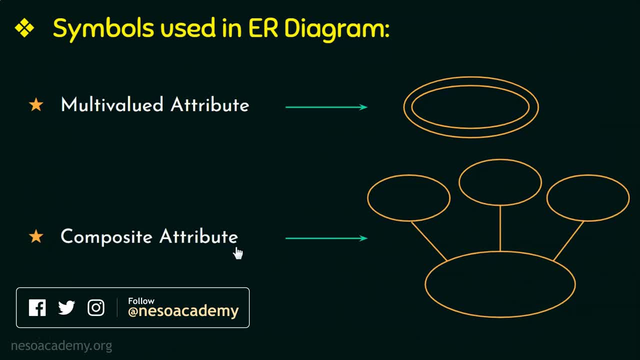 by double oval. Then we have the composite attribute, which is an attribute that can be divided into further attributes. Next is the derived attribute, which is an attribute whose value is derived from another attribute, and it is represented by a dashed oval. And finally, we have the identifying relationship. Earlier in this video, we have already seen what 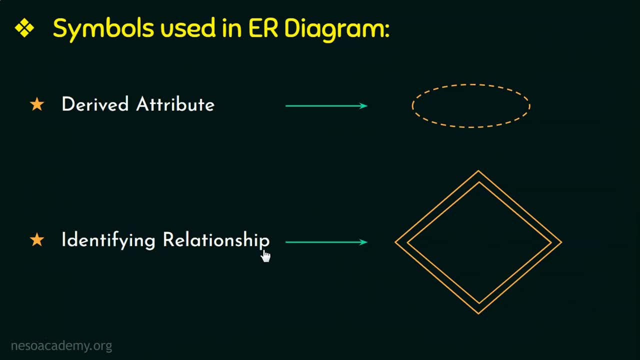 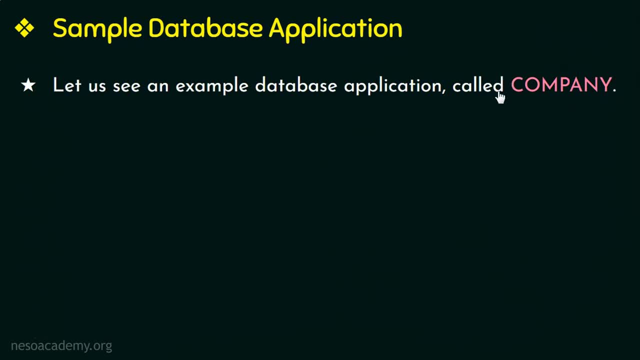 In this example, we already discussed what we call database application called company. In this example, we already discussed what we call database application called company. Here we have considered a company database, and a company database keeps track of the company's employees, departments, projects and dependents. 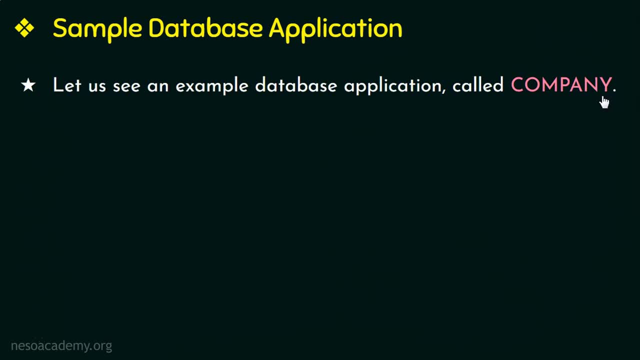 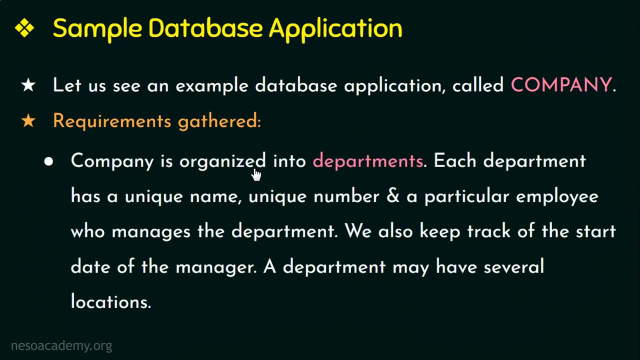 The first steps that we learnt in the database design process is requirements collection and analysis. So the requirements gathered are as follows: The company is organised into different departments And each department has a unique namespace. Each department has a unique namespace name, a unique number and a particular employee who manages the department. we 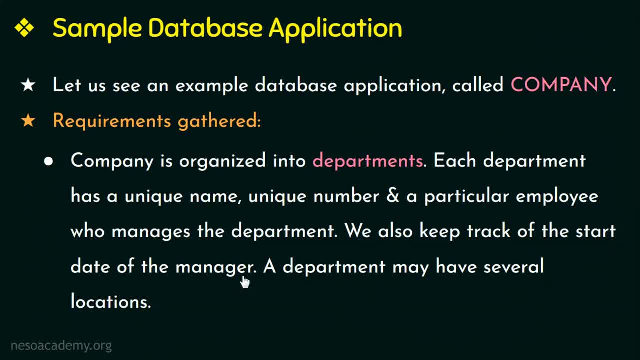 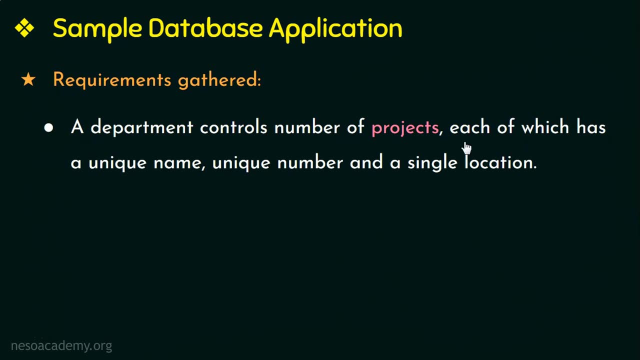 also keep track of the start date of the manager or the employee who manages the department, and a department may have several locations. this is one of the requirement. the next requirement is a department controls number of projects, each of which has a unique name, unique number and a single location. the next: 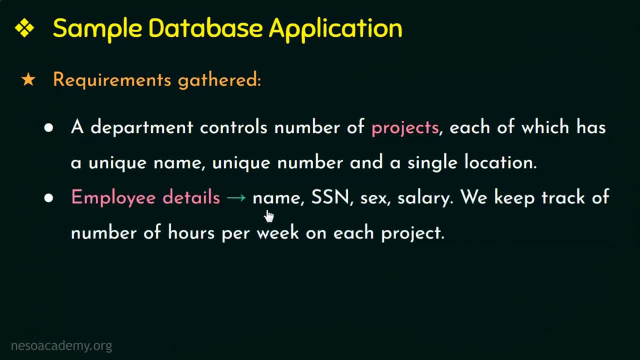 requirement is we store employee details like the employee name, the social security number, which is definitely unique for each employee, sex or the gender of the employee and salary details. we keep track of the number of hours per week an employee works on each project. we also keep track of each 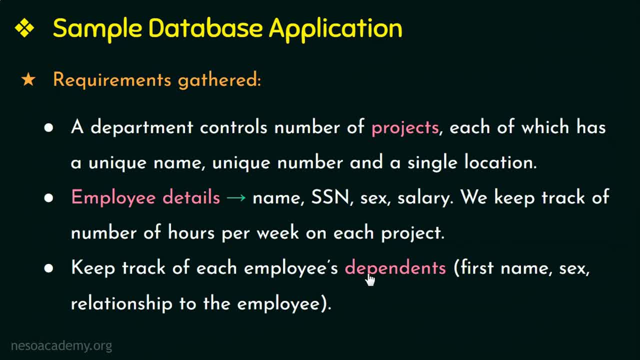 employees dependents. now, an employee's dependents could be their spouse, parents or children, or anyone that is working for the company is dependent on this employee. we need each dependents first name, sex and relationship to the employee. so these are the requirements gathered for the company database. the next step, after collection of requirements was 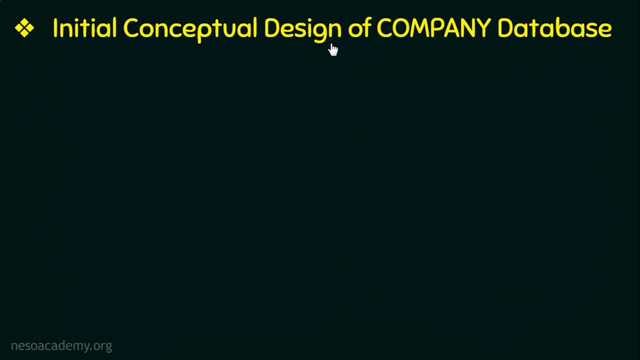 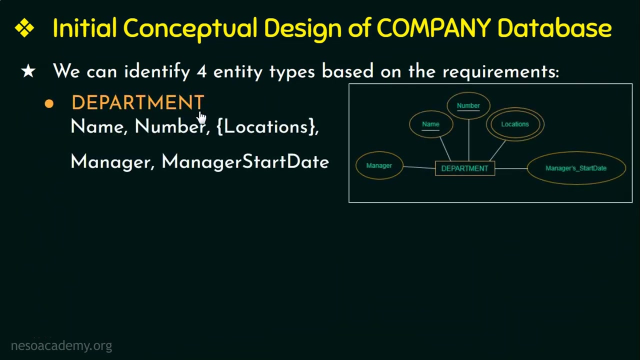 conceptual design. so, based on the requirements that we have gathered, let us see the initial conceptual design of the company database. we can identify four entity types based on the requirements that we gathered. the first entity type is the department. this entity type has attributes like the department name, department number, locations and employee who manages the 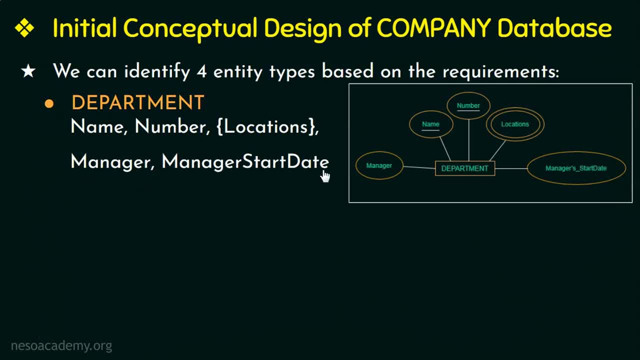 department, or otherwise called the manager, and the manager start date. since department can have several locations, this attribute is a multi-valued attribute and hence represented by a double OV. in our requirements, we have specified that the department name and number has to be unique and since they 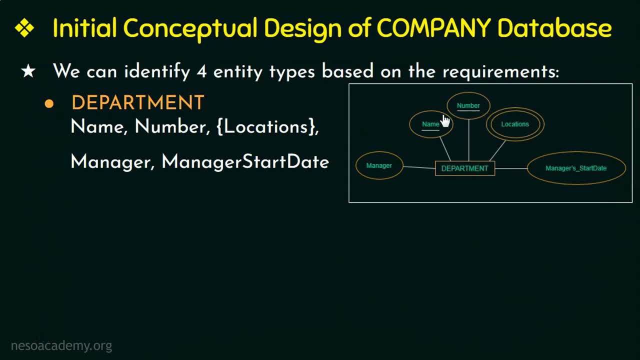 are unique. they are the key attributes of the department. so we need to identify the key attributes for this entity type, so either the department name or the department number can be a key attribute for this entity. the next entity type identified is project. this entity type has attributes: project name, project. 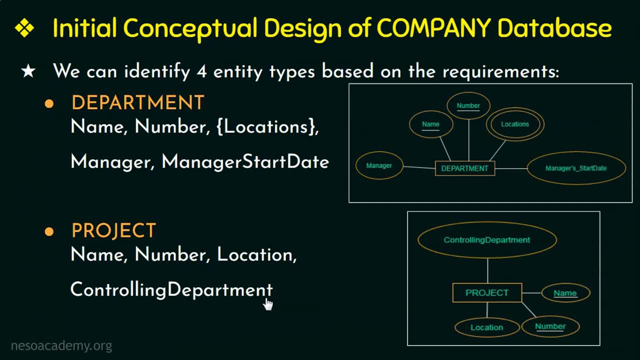 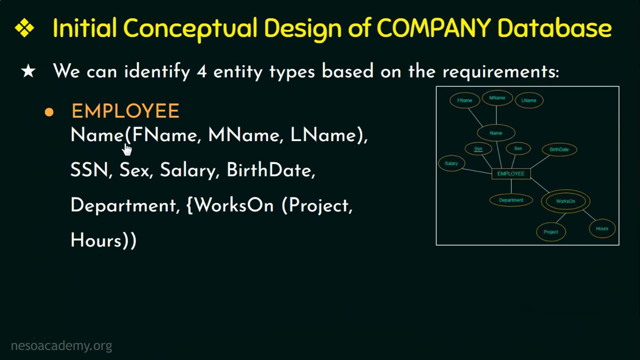 number, location and the controlling department, again based on the requirements. the project name and the number has to be unique, so any one of this can be a key attribute for this entity. the third entity type is a employee with attributes: employee name specifying the first name, middle name.